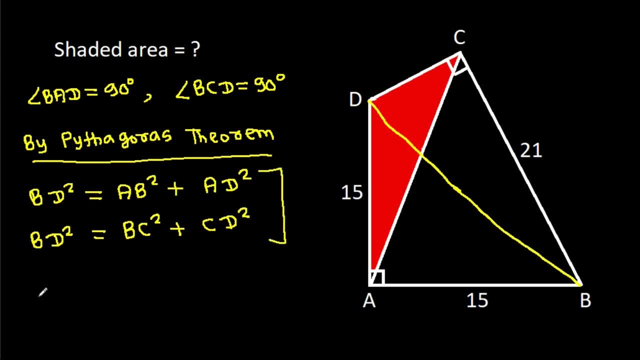 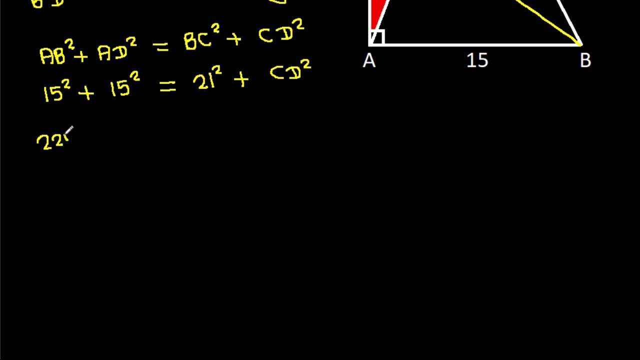 So from these two equations we can say that AB squared plus AD squared, it will be equal to BC squared plus CD square, and AB is 15 square plus AD is 15 square. it is equal to. BC is 21 square plus CD square, and 15 square is 225 plus 225. it is equal to 21 square. it is 441. 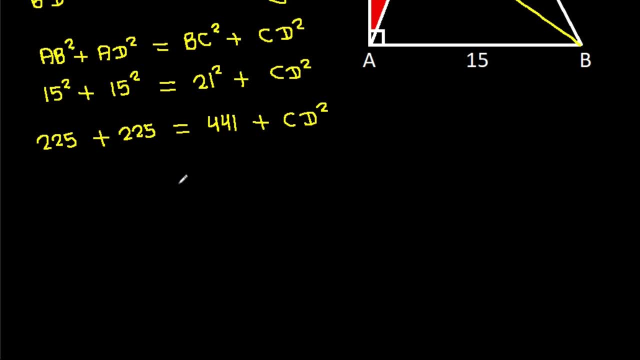 plus CD square and 225 plus 225 it will be 450. it is equal to 441 plus CD square. so CD square it will be 450 minus 441, and CD square it is 9, so CD square it is 9, so CD square it is 9, so CD. 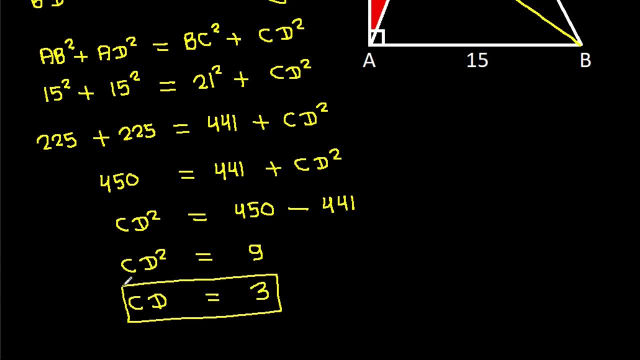 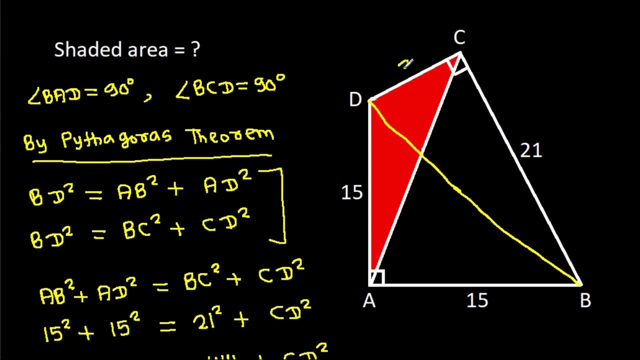 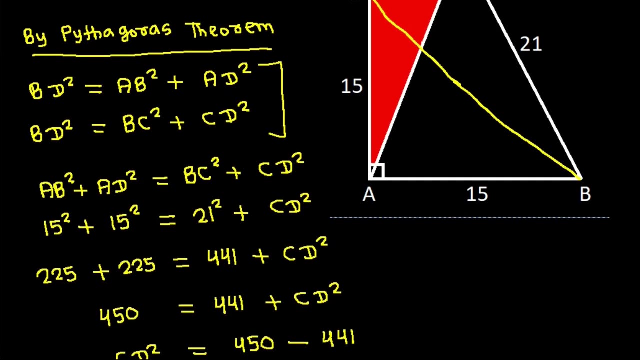 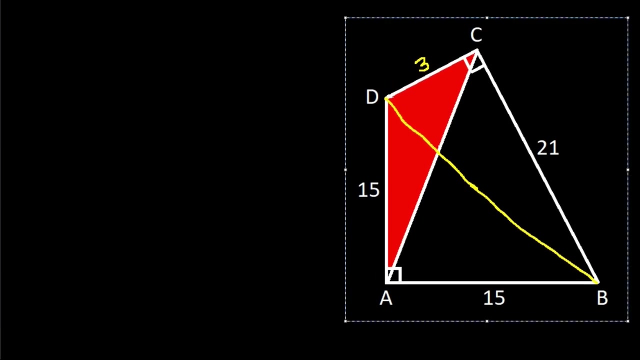 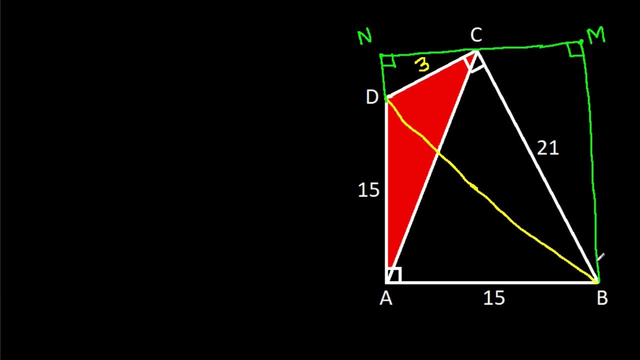 suppose this point is M and this point is in such that AB MN is in such that AB MN is in such that AB MN it is rectangle. it is our construction. now, if now, if this angle is 90 degree, so this angle it. this angle is 90 degree, so this angle it. 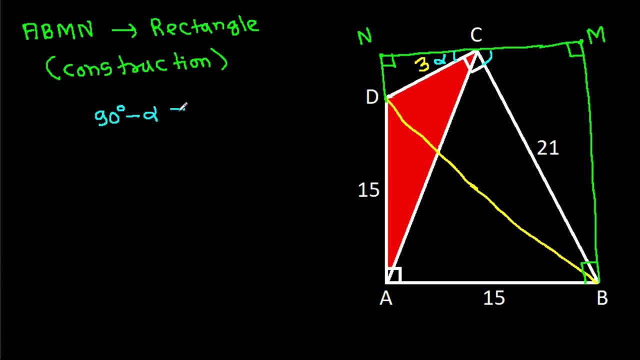 this angle is 90 degree, so this angle, it will be 90 degree. I am counting 90 and will be 90 degree. I am counting 90 and degree minus alpha. suppose it is beta, so it will be beta and this angle is 90. 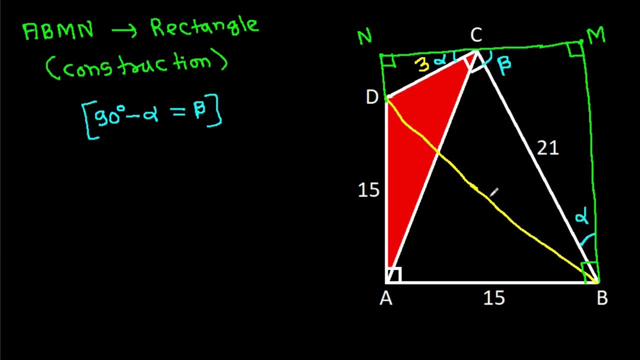 degree, so this angle it will be alpha. and here this angle is alpha, this angle is 90 degree, so this angle it will be beta. and now in triangle CDN and triangle BCM we have: angle CDN is equal to angle BCM, that is beta, and angle DCN it is: 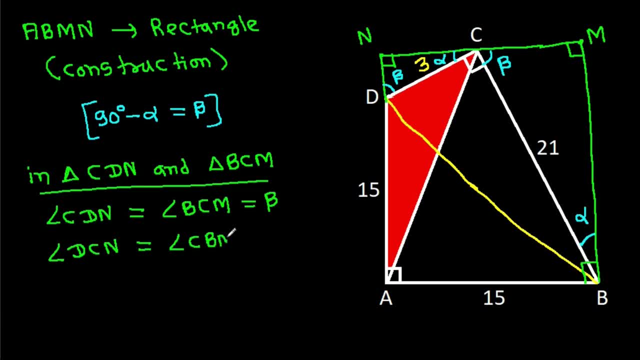 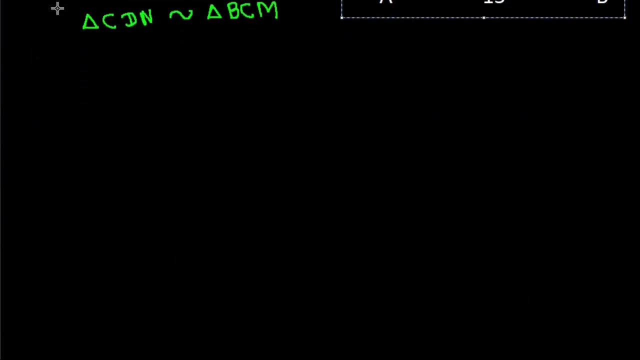 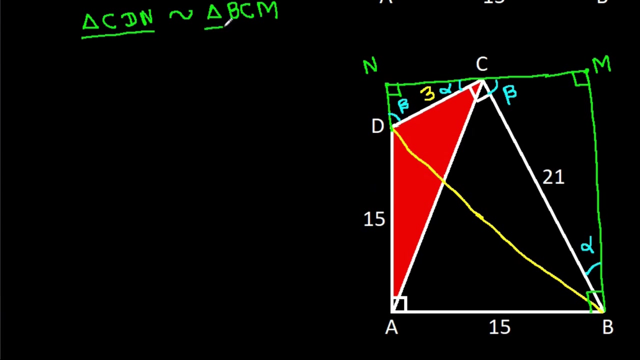 equal to angle CBM, that is alpha. so by angle, angle, similarity, angle CDN, it won't be similar to terangle BCM and these two terangles are similar, hence CD by BC it will be equal to DN, by CM it will be equal to CN by BM. and we have: CD is 3, by BC is 21 it. 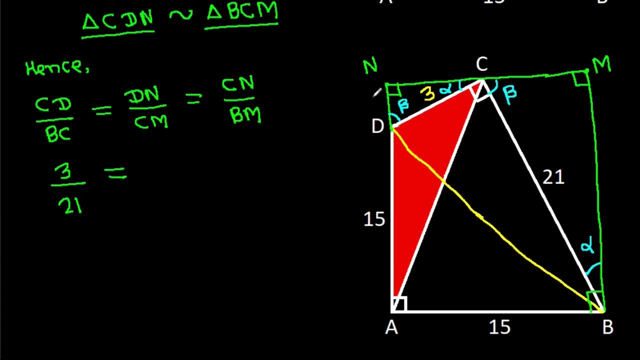 is equal to, and suppose DN is A by and suppose CM is B, it is equal to. and now we know that ABMN it is rectangle, so AB is 15, that means MN it will be 15, and MC is B, so CN it will be 15 minus B. 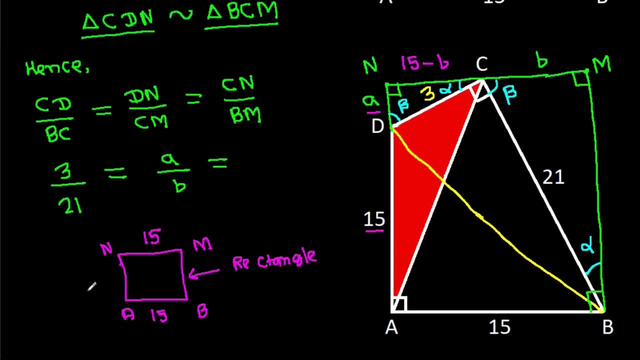 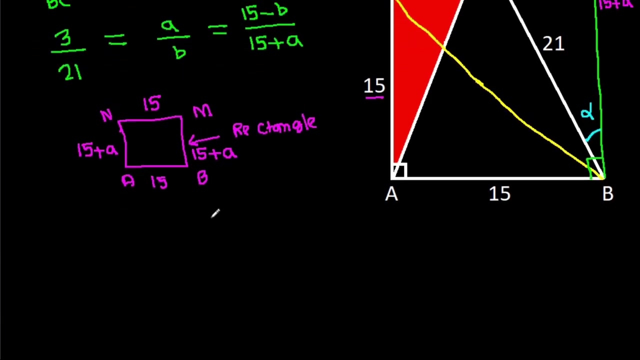 and AN it is 15 plus A. AN is 15 plus A, so BM it will be also 15 plus A. BM it will be 15 plus A, so CN it is 15 minus B. by BM it is 15 plus A. so we get: 3 by 21 is A by B, and we get: 3 by 21 is 15 minus B by 15. 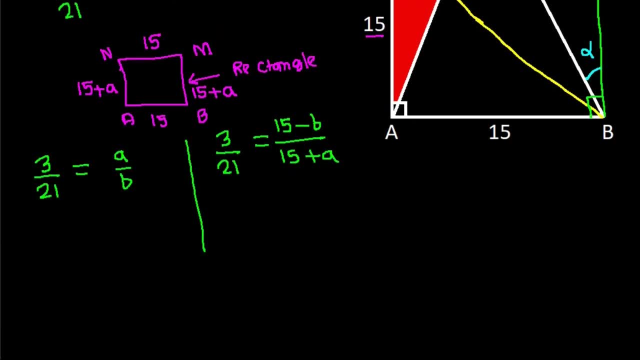 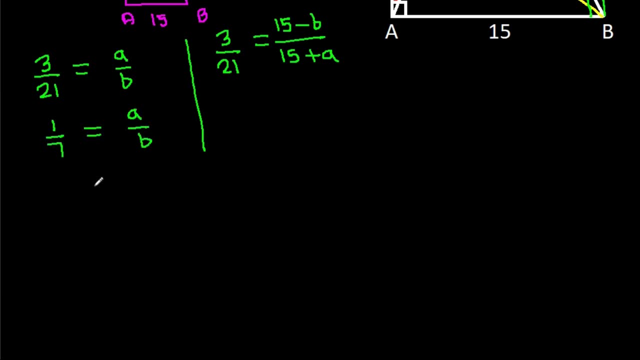 plus A. And from here we get: 1 by 7 is A by B, so B will be equal to 7A. and from here we get: 1 by 7 is 15 minus B by 15 plus A, and if we cross multiply then 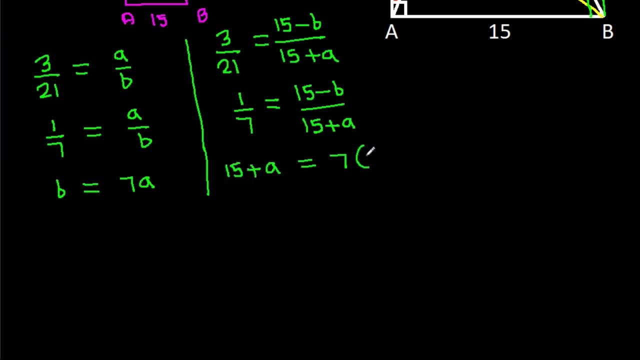 then 15 plus a, it will be 7 times 15 minus b, and 15 plus a it is equal to 105 minus 7 b, and it is 15 plus a is equal to 105 minus 7 times b is 7 a and 15 plus a it is 105. 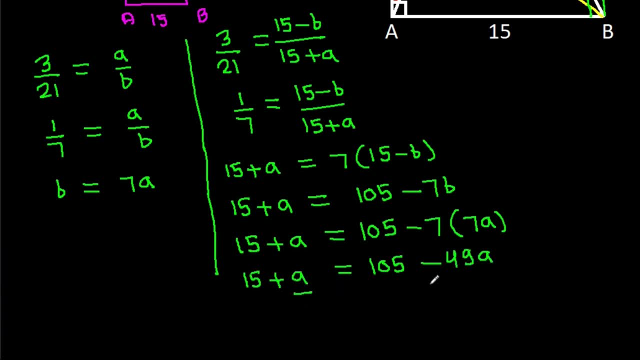 minus 49 a and a plus 49 a, it will be 50. a it is equal to 105 minus 15, it will be 90, and 0 will get cancelled. so a will be equal to 9 by 5.. and b will be equal to 7 times a is 9 by 5, so b will be equal to 63 by 5.. 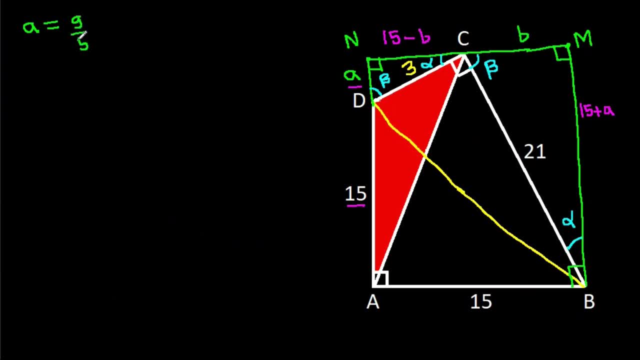 We get: a is 9 by 5 and b is 63 by 5. and now inter angle a d c, it is a d c, it is a d c c. a d is 15, so area of a d c it will be 1 by 2 times base times height. and it is 1 by 2 times base is a d and height it is c? n. 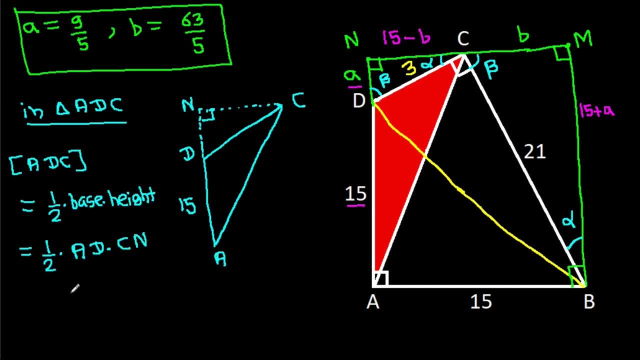 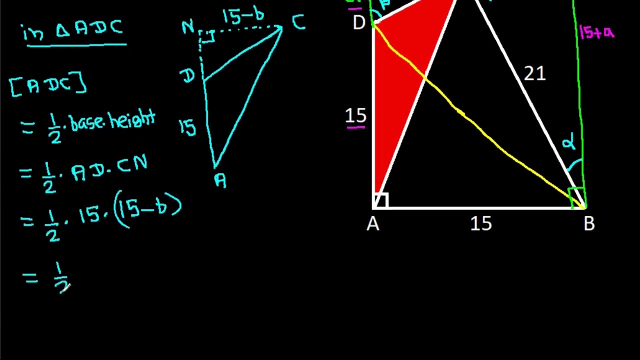 Height is c? n and it is 1 by 2 times a? d is 15 and c? n is 15 minus b. c? n is 15 minus b and it is 1 by 2 times 15 times 15 minus b. 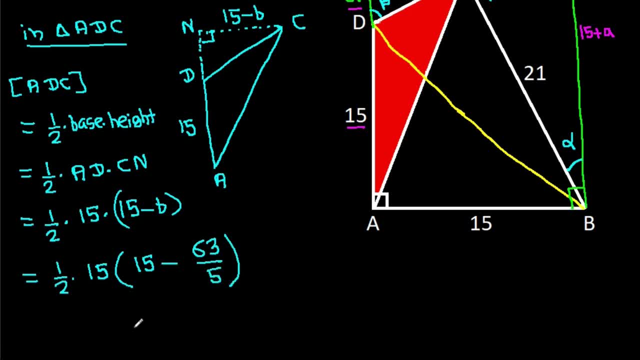 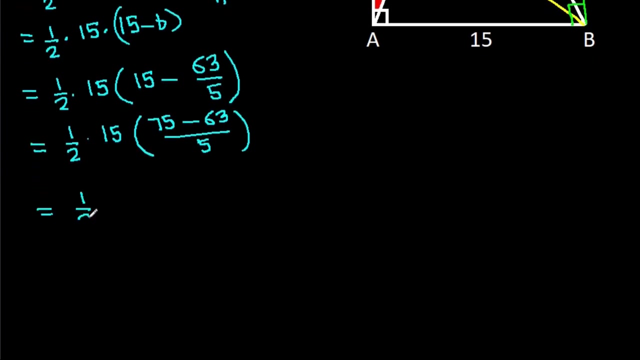 b is 63 by 5, and it is 1 by 2 times 15 times 15 times 5 is 75 minus 63 by 5, and it is 1 by 2 times 15 times 12 by 5..